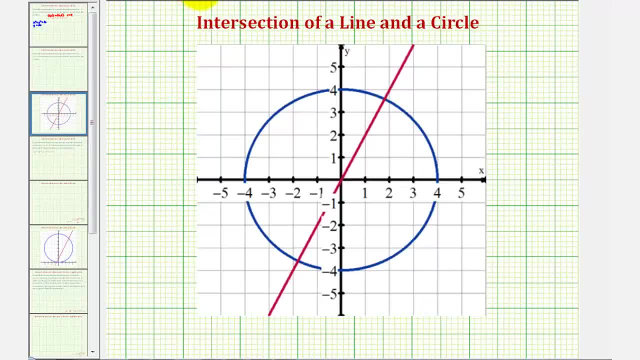 look at the graph of the circle and the line. Notice how the circle is centered at the origin with a radius of 4, giving us the equation x squared plus y squared equals 16.. And the given linear equation was y equals 2x. so notice how the y 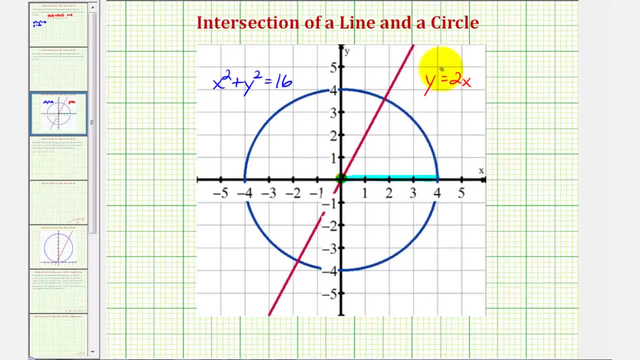 intercept of this line is 0 here and because the slope is 2 or 2 over 1, notice, if we go up 2 and right 1, we find another point on the line. And because we're looking for the point of intersection in the first quadrant, we're 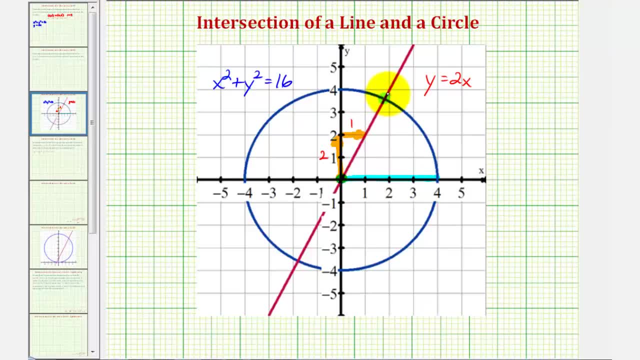 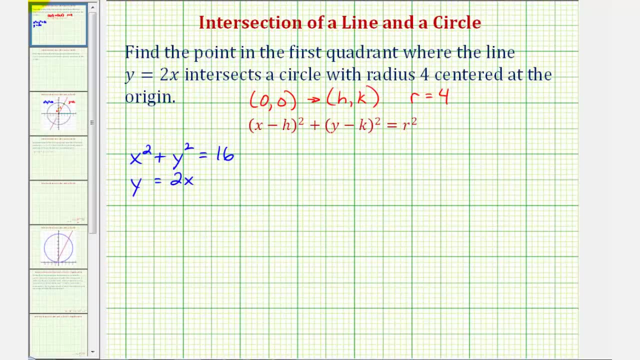 looking for this point here. So, going back to our system of equations, let's solve this using substitution, where, if y equals 2x, we'll substitute 2x for y in the first equation. This will give us an equation with just x. We would have x squared plus instead of y squared we'd have 2x. 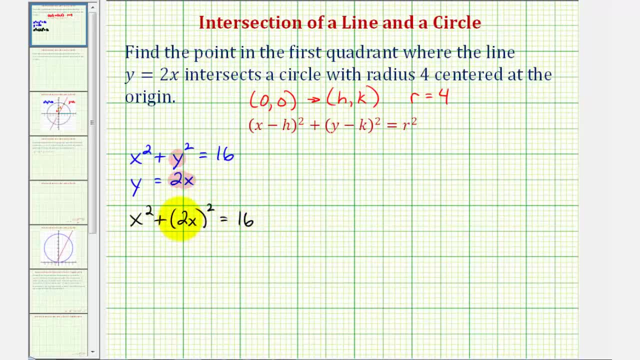 squared equals 16.. 2x to the second power would be 4x squared. so we have x squared plus 4x squared equals 16.. x squared plus 4x squared, or 1x squared plus 4x squared, would be 5x squared. 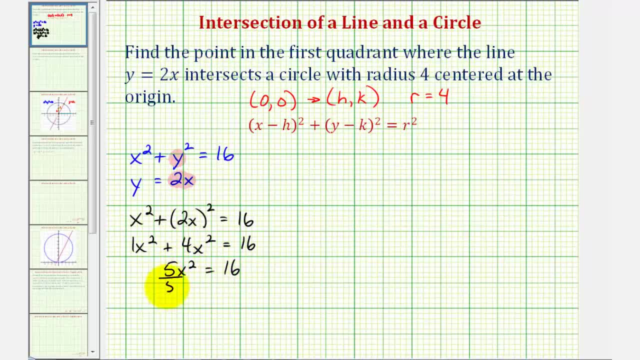 Isolate x squared by dividing both sides by 5.. So we have: x squared equals 16 fifths. Notice here: x can be both positive or negative. So now, when we take the square root of both sides of the equation, we need to be sure to include a plus, or 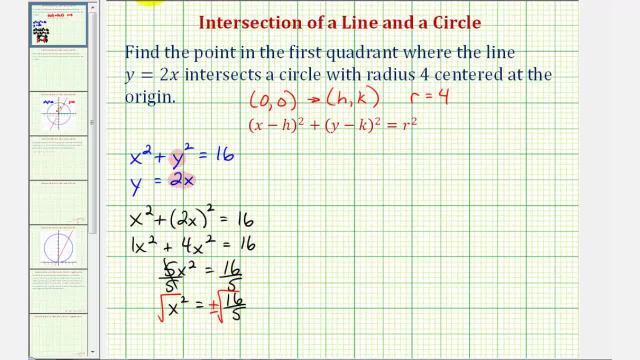 minus sign on the right to obtain both solutions. So we have x equals plus or minus the square root of 16 divided by the square root of 5.. But since the square root of 16 is equal to 4, we have x equals plus or minus 4 divided by the square root of 5.. Now, because we're 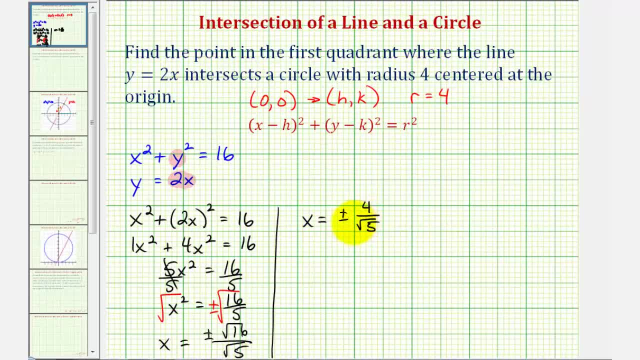 looking for the point in the first quadrant, we know x has to be positive. So for our purposes, we know that x can only be positive: 4 divided by the square root of 5.. Now you may be asked to rationalize this, but we'll show that in a few moments. Right now we just found that the point of 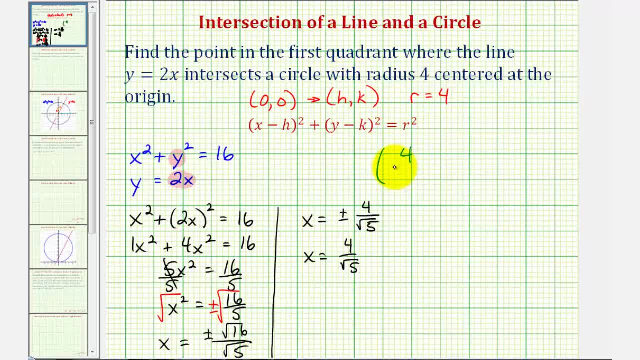 intersection in the first quadrant has an x coordinate of 4 divided by the square root of 5.. Now let's find the y coordinate of the point of intersection. Well, we know y must equal 2 times x, or y equals 2x. So if 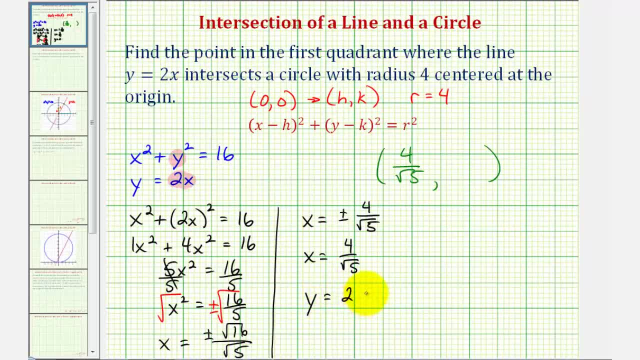 y equals 2x, and now we know the value of x. we can find y. y would be equal to two or two over one times four divided by square root of five, which would be eight divided by square root of five. 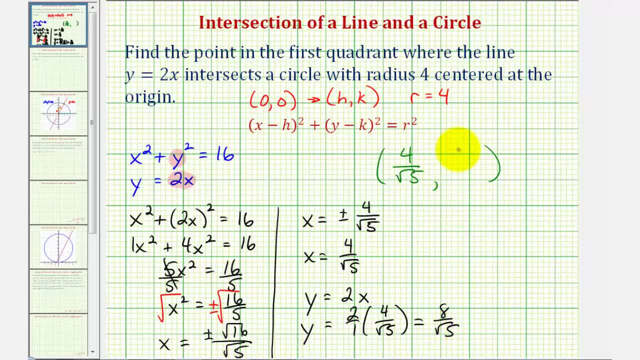 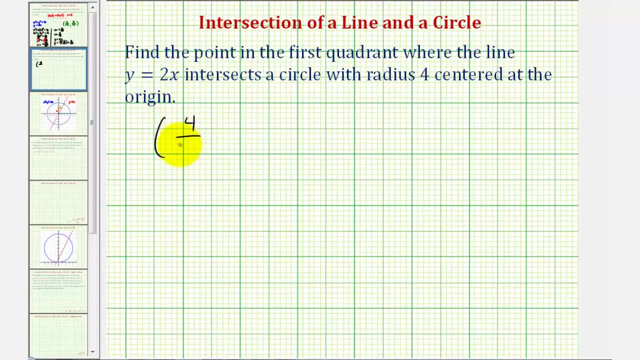 So this would be the y-coordinate of the point of intersection in the first quadrant. Now I'll show how to rationalize these coordinates and also how to get a decimal approximation. So again, we just found the x-coordinate is four divided by square root of five. 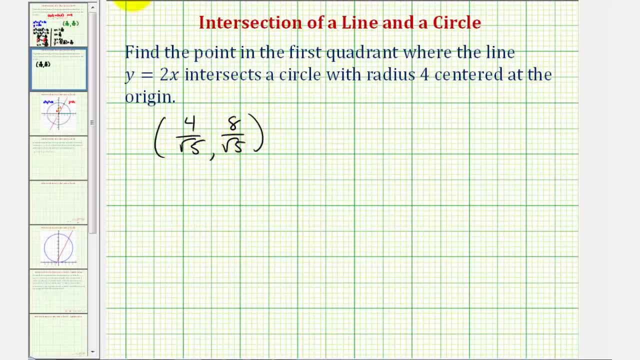 and the y-coordinate is eight divided by square root of five. So if we want to rationalize four divided by square root of five, we'd have to multiply the numerator and denominator by square root of five, which would give us four square root of five. 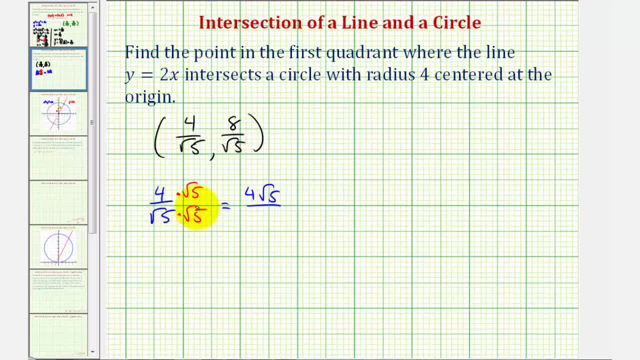 divided by square root of five times square root of five, which is a square root of 25, or just five. So again this was x And then y. remember? y is equal to two times x, so two times one times four, square root of five over five. 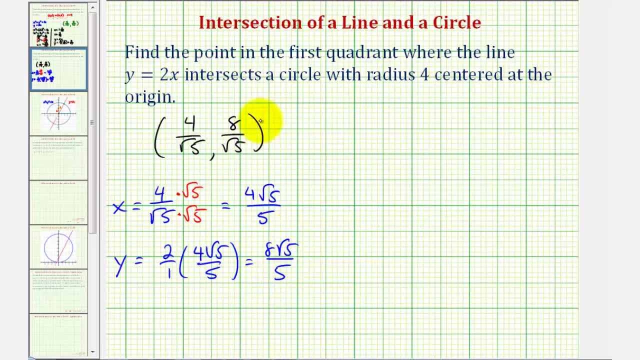 would just be eight square root of five over five. So if we are required to rationalize the denominators of these coordinates, we would say four square root of five divided by five, comma: eight square root of five divided by five. And also, just in case you are asked to round these values: 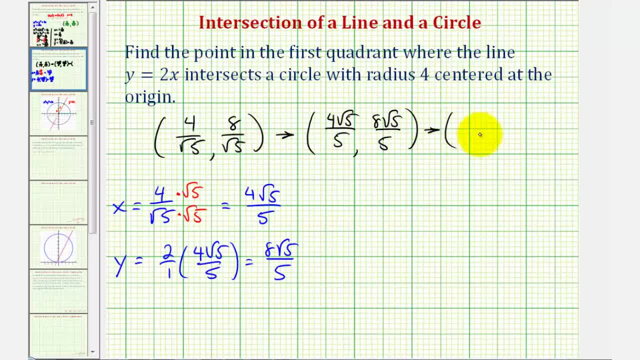 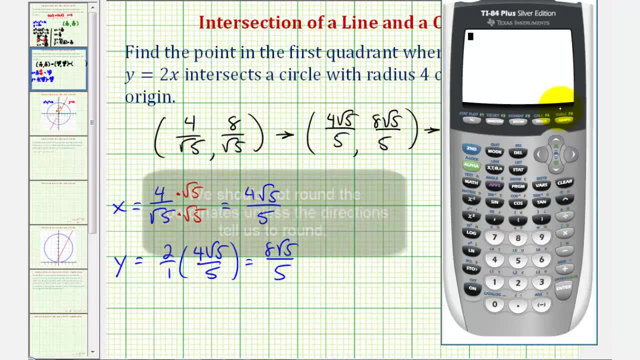 to, let's say, three decimal places. let's also show that Of course this would require a calculator and it would be easier to use these coordinates to convert to a decimal. So to convert the x-coordinate to a decimal we would have four divided by.